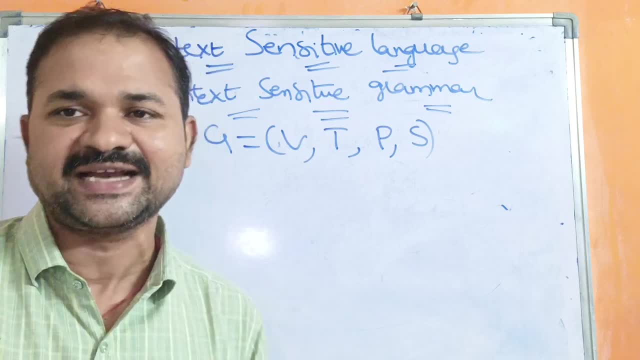 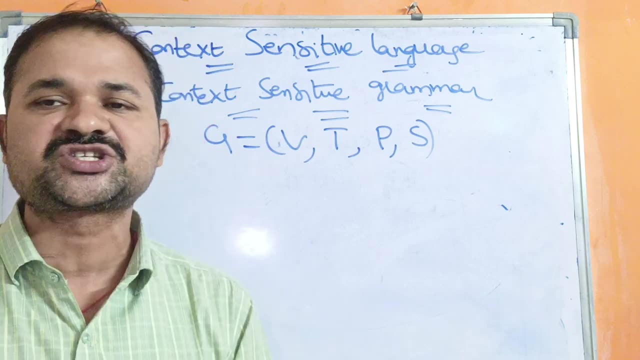 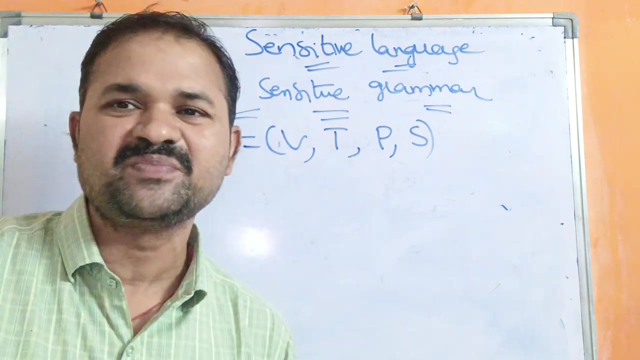 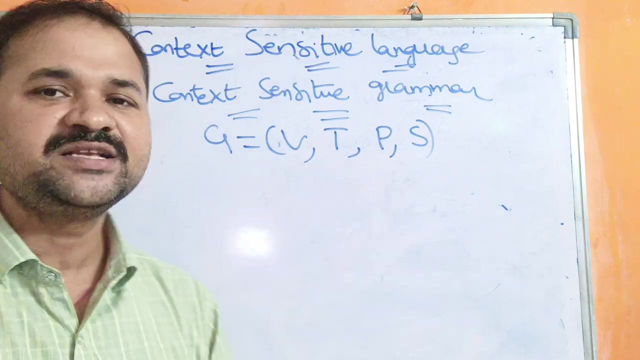 Variables or non-terminals are represented by uppercase letters. T means set of terminal symbols. Terminals are represented by lowercase alphabets. or we can use digits from 0 to 9, or we can use combinations of digits, some numbers, 10, 20, 30, likewise also. Or terminals mean symbols, also Plus, minus, star likewise. P means a set of production rules, S means starting symbol. 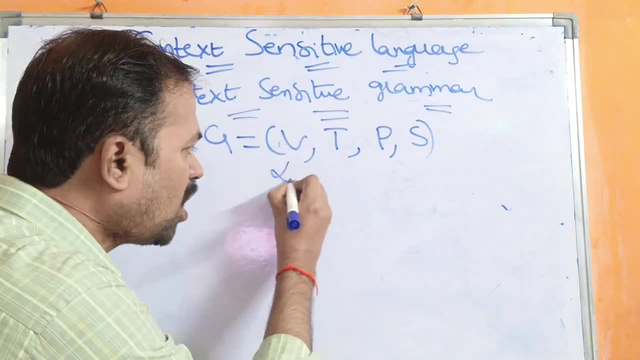 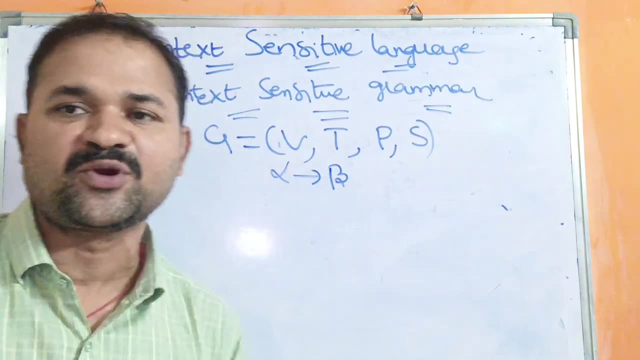 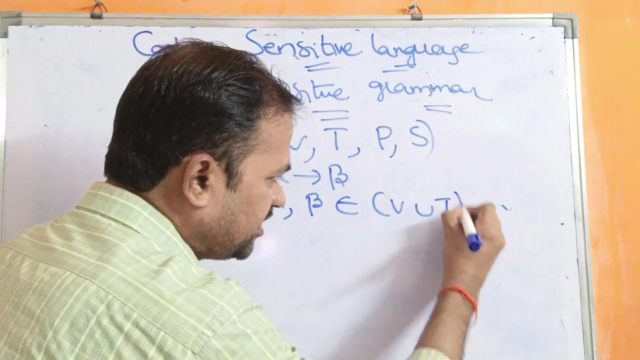 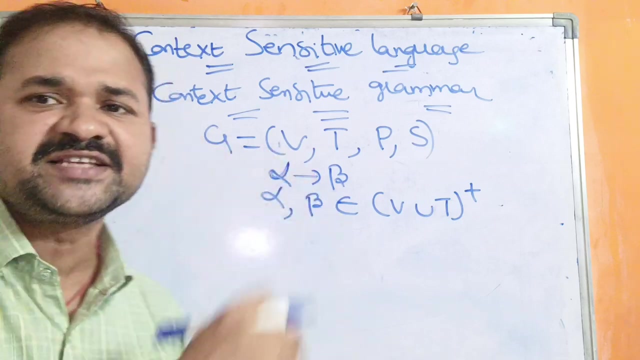 Here the productions are of the form. alpha implies beta. Alpha means left-hand side production. Beta means right-hand side production. Here the productions contains a combination of variables and terminals. Variables and terminals: Here alpha means left-hand side production. Left-hand side should contain minimum one, non-terminally. 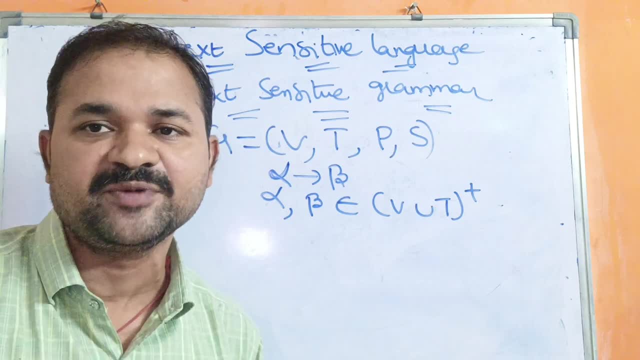 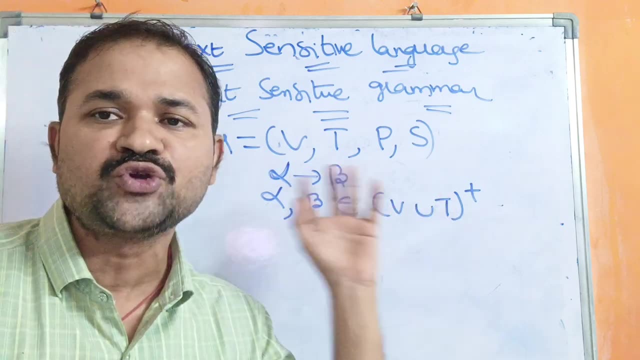 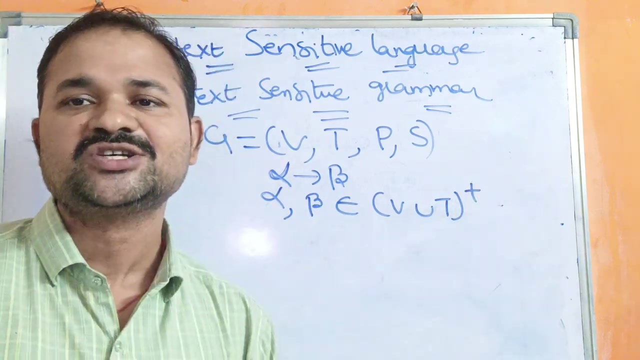 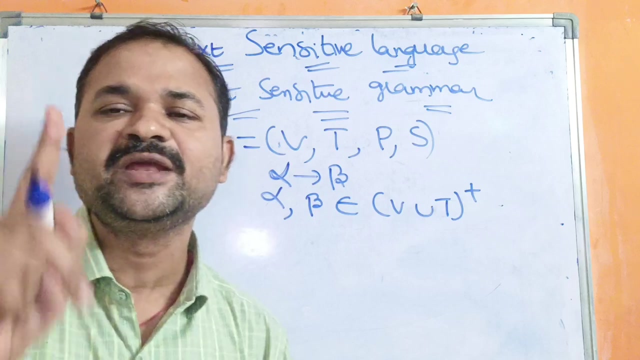 Right-hand side should not contain epsilon. So that's why here we have written plus. That's why here we have written plus. So star means any number of occurrences, including zero occurrences. also, Where he has plus means minimum one occurrence. So here alpha and beta are a combination of variables. 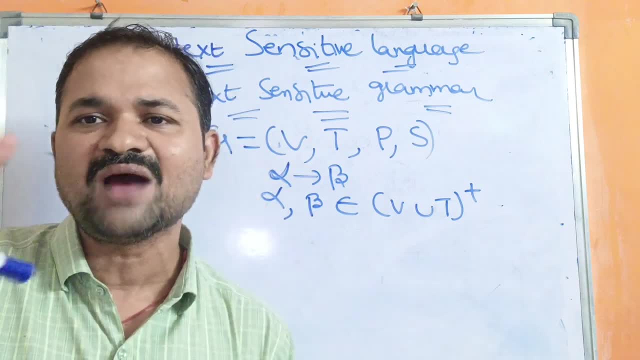 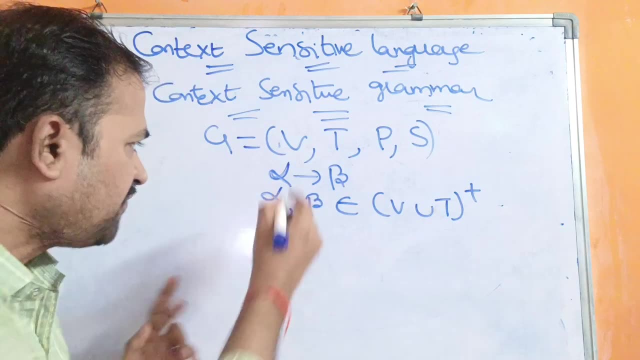 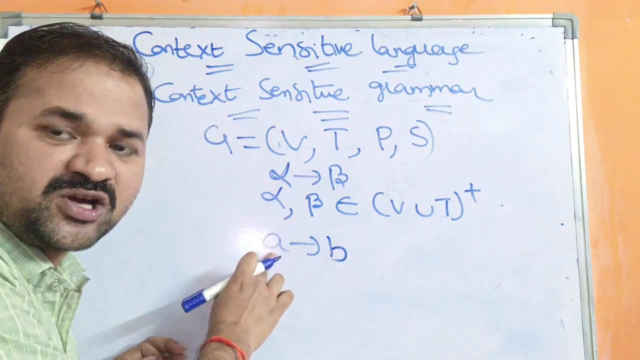 Variables and terminals. But we have two conditions: Alpha, That means left-hand side production- should contain minimum one non-terminal. So left-hand side production should not be like this. A implies B. Why? Because here left-hand side production is a terminal symbol. 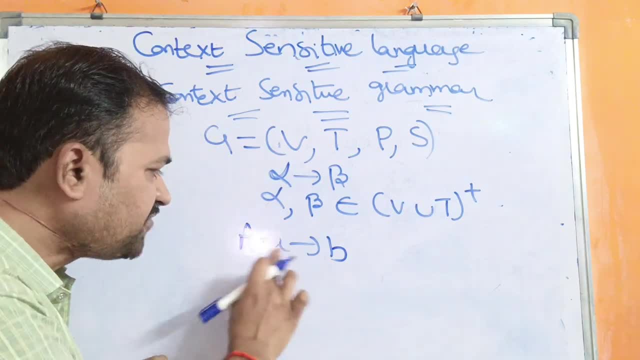 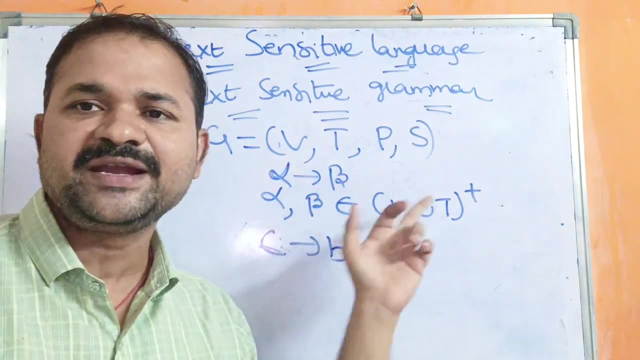 We have a production like this: A A Okay, And left-hand side production, and right-hand side production should not contain epsilon. Okay, And what is the second condition For beta? the condition is the right-hand side production, that is, beta should not contain epsilon. 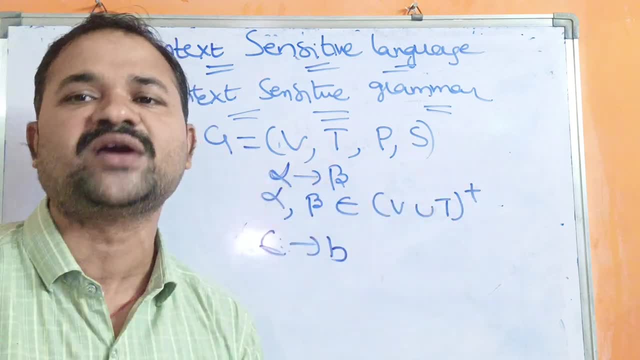 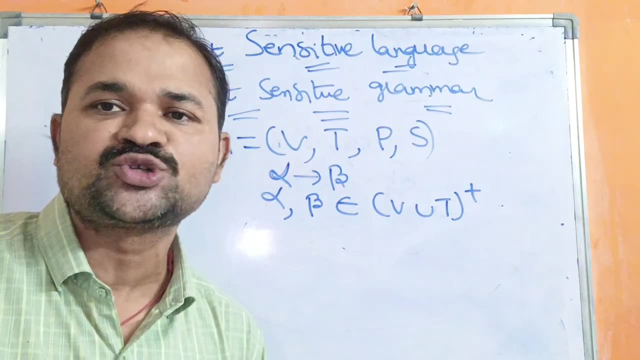 So that's why here we have written plus. So plus means minimum one occurrence. So left-hand side should contain minimum one non-terminal, as well as left-hand side should not contain epsilon. Next, right-hand side should not contain any epsilon. Okay, 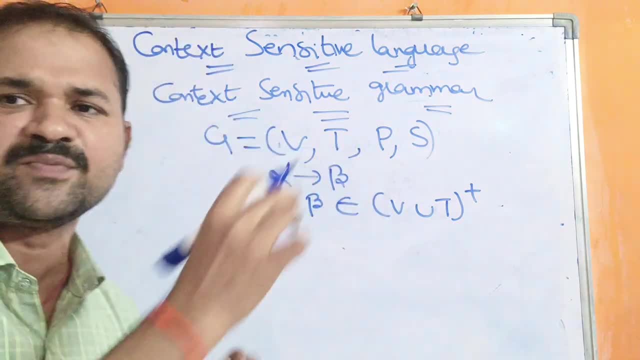 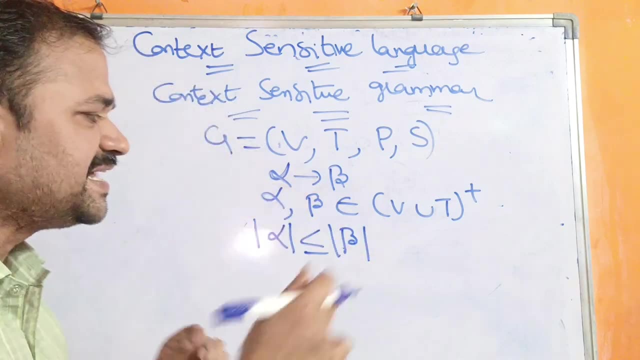 Let us see some examples here. And we need to follow one more condition Here. mod alpha is less than or equal to mod beta. Mod alpha is less than or equal to mod beta. So mod means length of the string. length of the alpha. 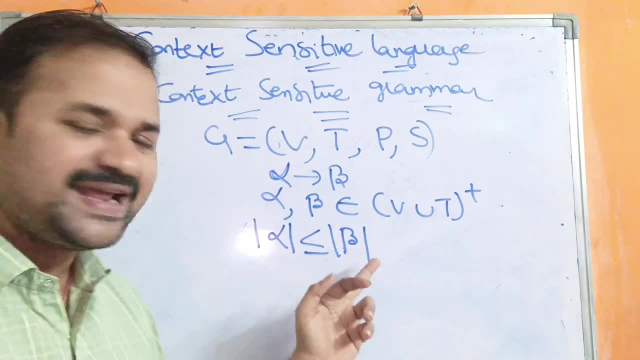 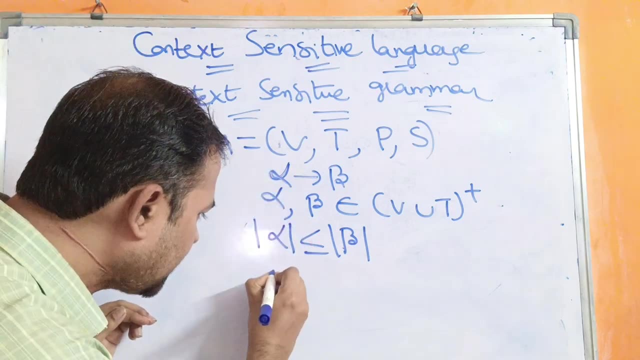 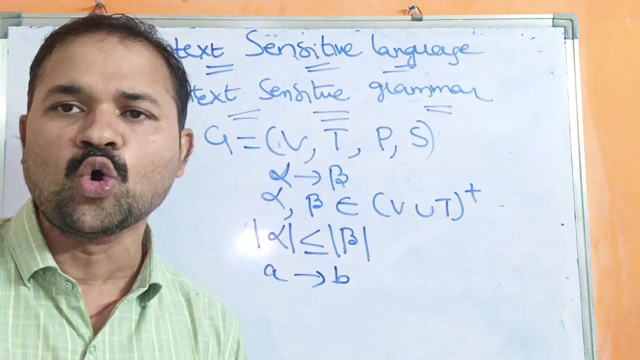 So length of the left-hand side production should be less than or equals to length of the right-hand side production. Okay, Let us take some examples. Let me have a production like this: A implies B. Is it a context-sensitive grammar? No, Why? Because context-sensitive grammar means left-hand side should be a non-terminal. 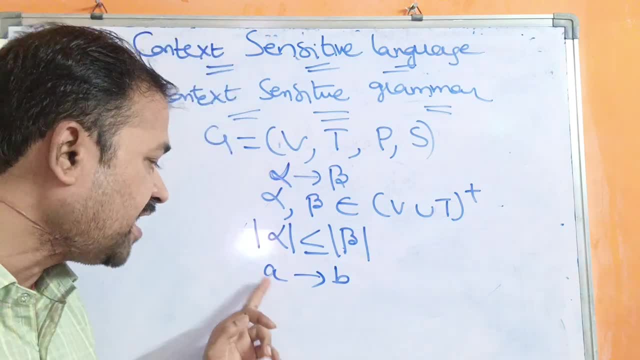 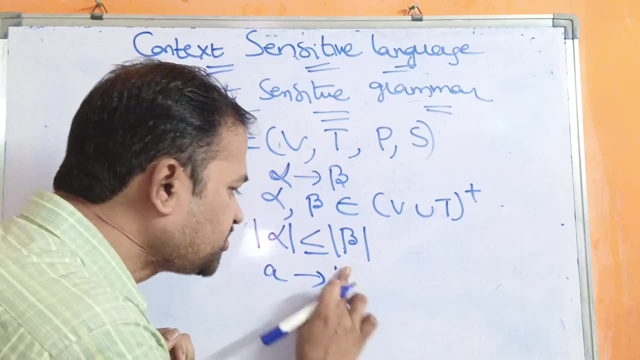 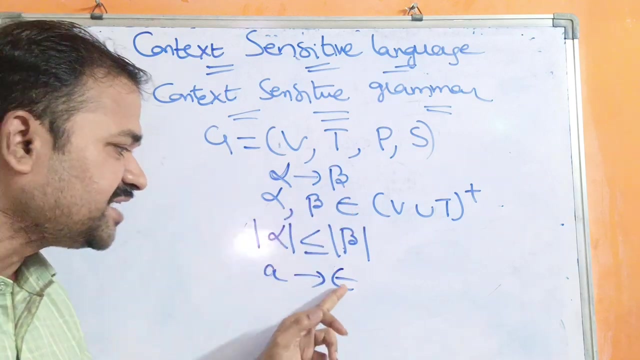 Left-hand side should contain minimum one non-terminal, But here we have only. but here we don't have any non-terminal. That's why this is not a context-sensitive grammar. Next, A implies epsilon. Is it a context-sensitive grammar? No, Why? Because right-hand side or left-hand side should not contain epsilon. 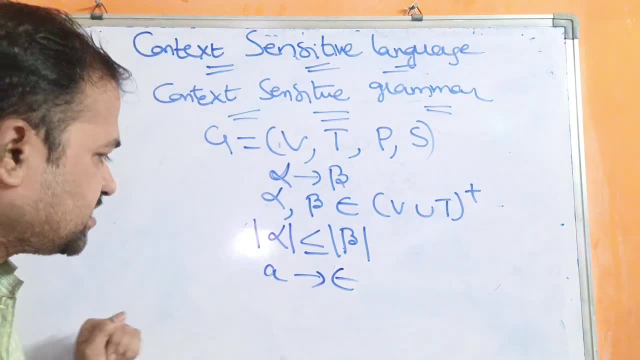 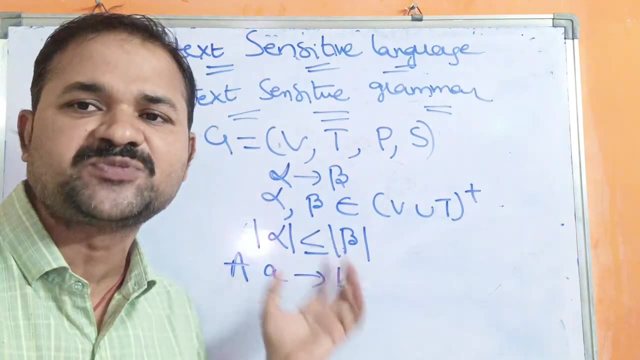 But here we have epsilon. Okay, So this is not a context-sensitive grammar. A implies A implies B. Is it a context-sensitive grammar? Is this: production is in CSC? Yes, Why? Because left-hand side contains combinations of terminals and non-terminals. 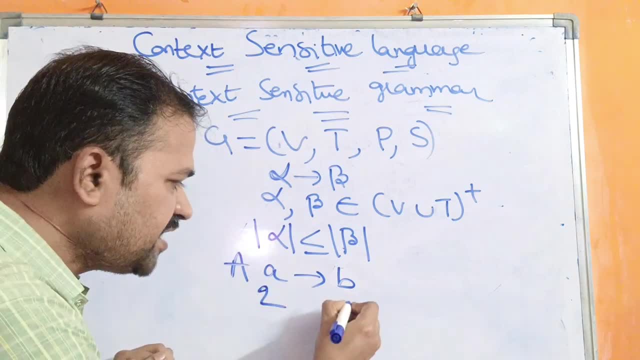 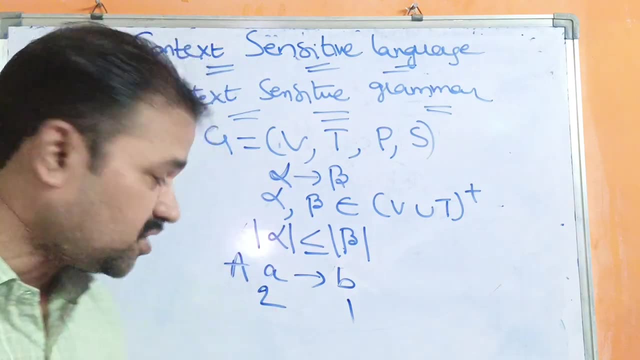 And what is mod alpha? Mod alpha means two. Variance, mod B means one, two. So two is less than or equal to one. Two is less than or equal to one Condition is false. So this production is not in, not in CSC. 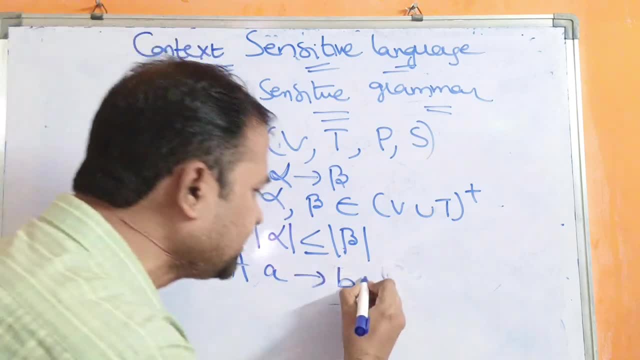 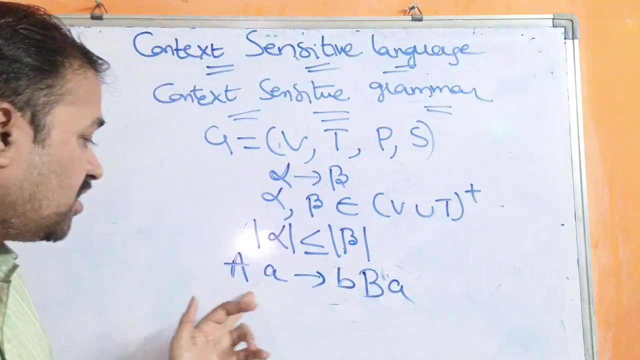 Okay, So if we want to make this here CSC, then let us add some more productions: A, B, A, So is this production is in CSC? Yes, Why? Because length of alpha is two Variance length of beta is three. 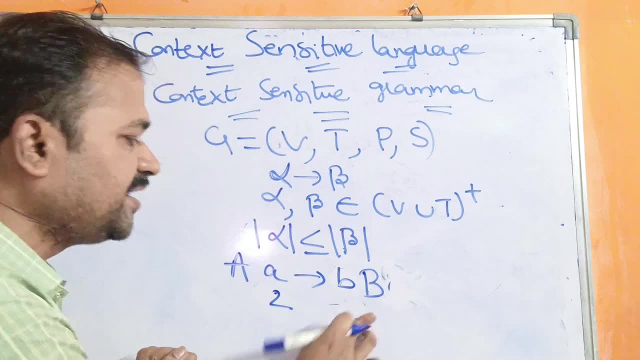 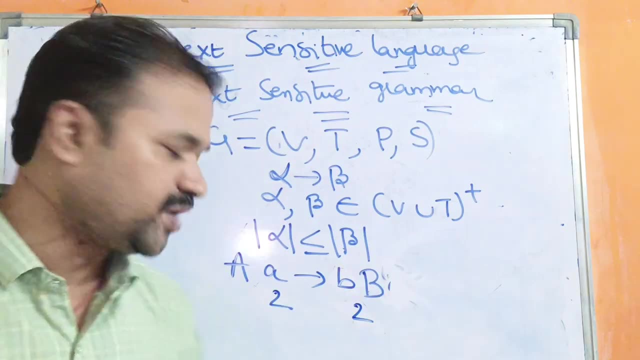 So two is less than three. The condition is true. So this is also in this production is also in CSC. Why? Because length of the left-hand side production is two, Length of the right-hand side production is two. Okay, Next is: this production is in CSC No.